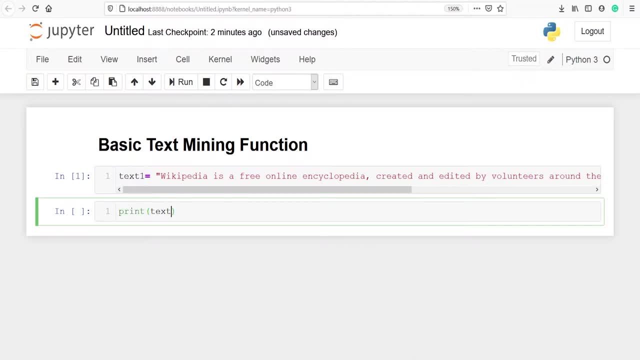 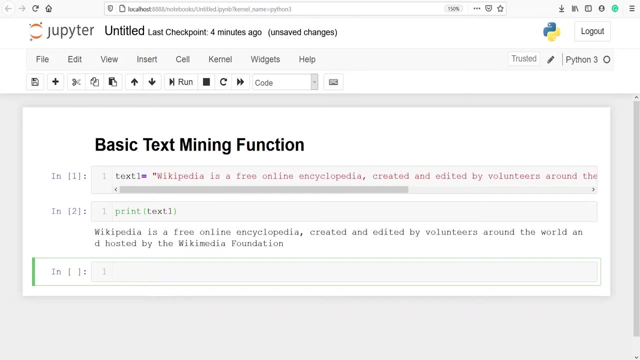 variable text1.. Print text1.. This is our text1 and this is a sentence. Let's look at the length function. Length function will tell you how many characters are there in the string. I will call the method length, Then I will pass our variable text1.. In the 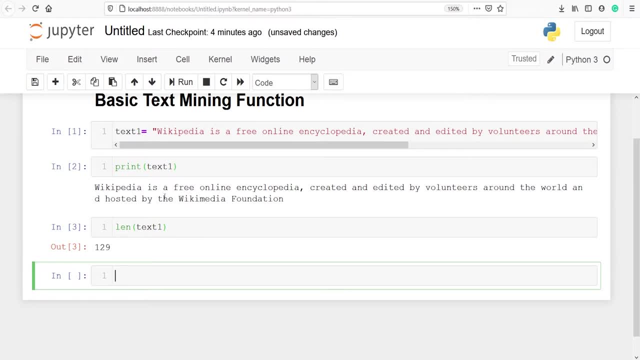 output we can see that we got 129.. Our variable text1 contains total 129 characters. The next method is split. Split methods will split the sentence into words. I will make one variable text2.. Here we can see we have a complete sentence and using the split method. 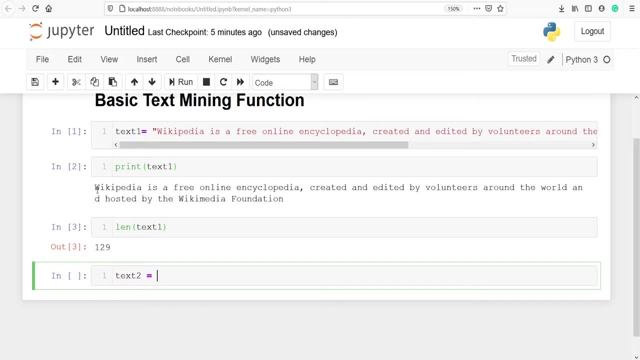 we will break this sentence into words. So the first word will be wikipedia, second will be is, third will be a and so on. Now I will call our variable text1.. Then I will call the methods split, And I want to split it on space, So I will type here single quotes and a space. 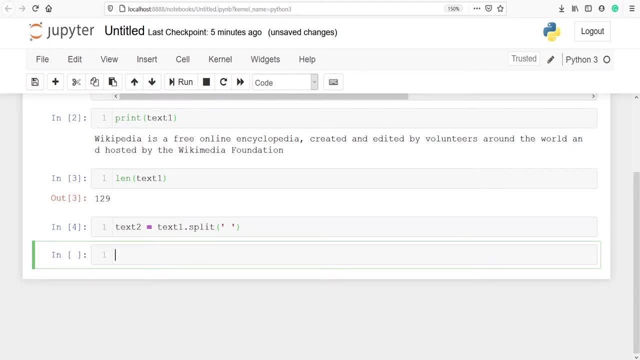 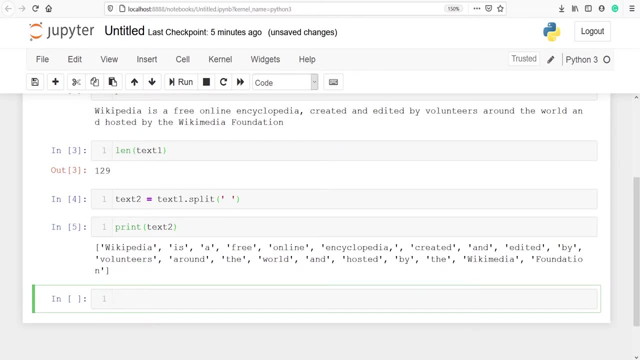 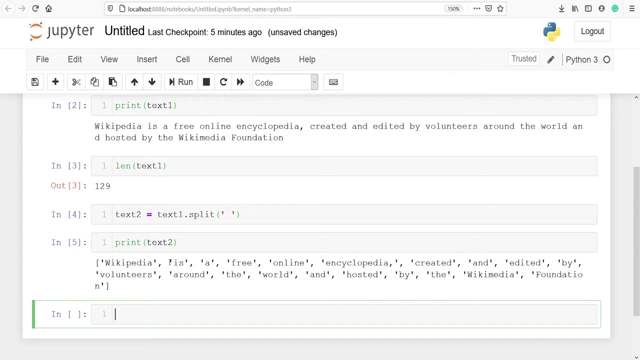 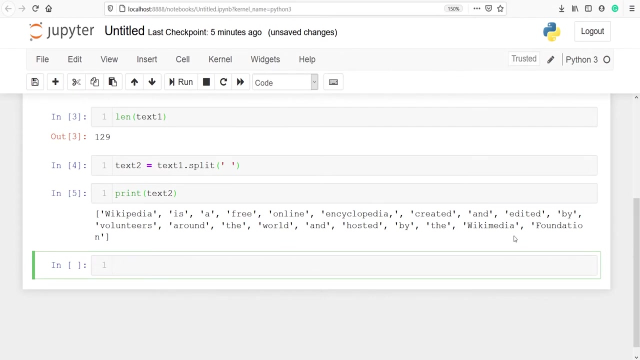 Let's execute our code Now. let's print our variable text to here. you can see that we have split our sentence into words. now. First we have Wikipedia, then is a free online, And so on. We can also find the number of words or tokens in the sentence. tokens are same. 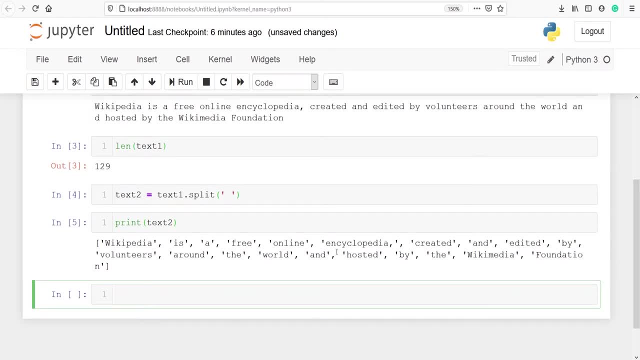 as words. we can call it words or token. So we want to count the number of words that are present in our variable text to. we will use the method length, l e, n. then we will call this variable text to and let's execute our code. There are total 20 words we can. count 1,, 2,, 3,, 4,, 5,, 6,, 7,, 8,, 9,, 10,, 11,, 12,, 13,, 14,, 15,, 16,, 17,, 18,, 19, and 20.. There are total. 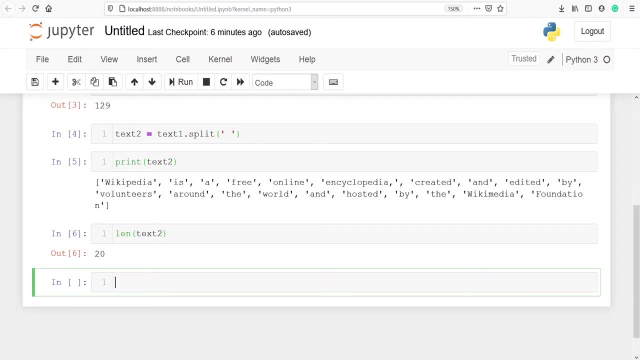 20 words in our variable text to. we can also find a specific words. For example, we want to find words that are more than four letters long. we will use the list comprehension. So here we will see. this word is middle, Made up of character And this word is made up of four character. You want to find ones? 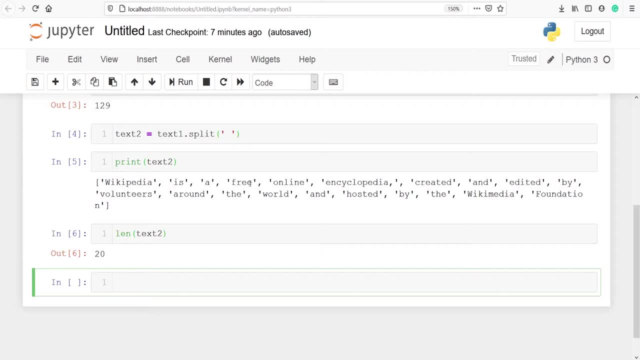 that are more than that, are made up of more than four characters, And make a right one, list comprehension, And I will write w for w in X, two, And then I will write the condition if length of w is greater than four. here I am saying that I am running a for loop and I am saying that if the length of words 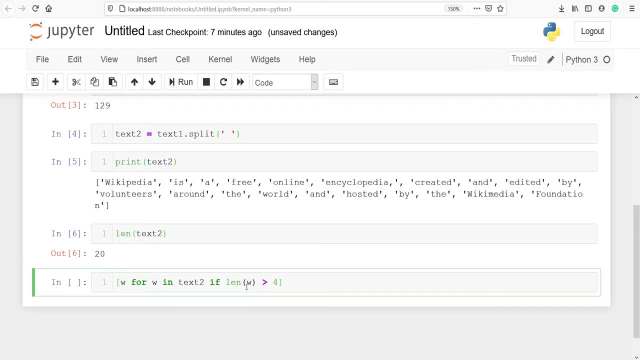 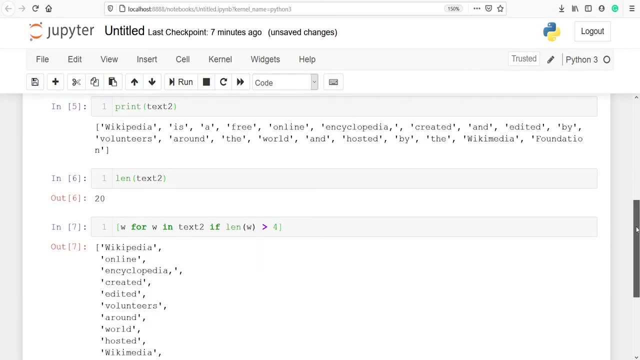 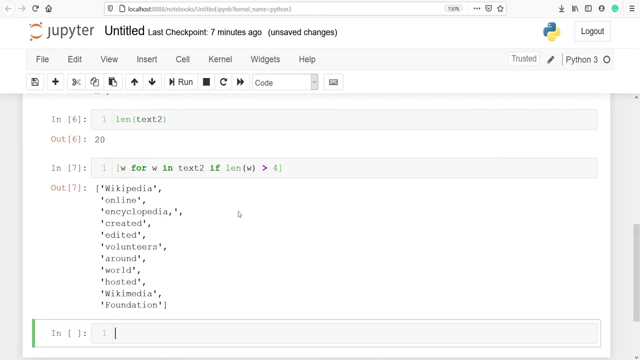 which are present in this variable text2 are greater than 4, then only print those words. I will execute the code and in the output you can see that we got some words here and all these words have a length greater than 4 and similarly, if I say less than 4, if I 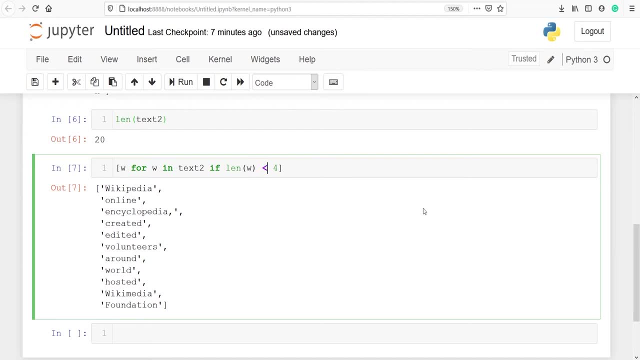 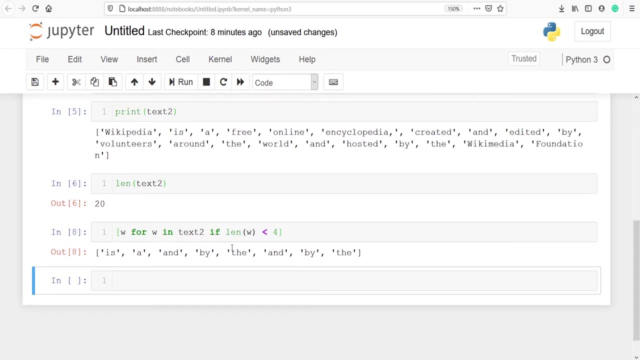 write the less than symbol here. now I will execute the code. in the output we got all the words that are of length less than 4, and these are a and bythe. so you can see here that all the words are less than the 4.. 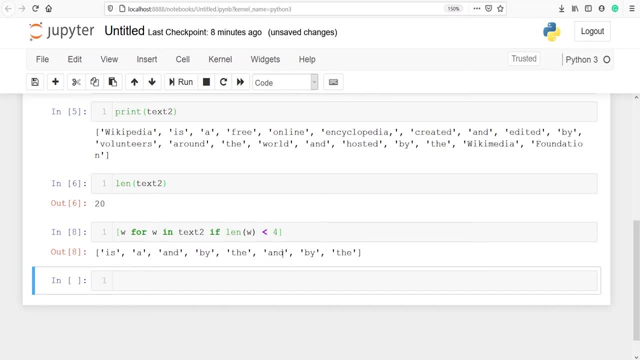 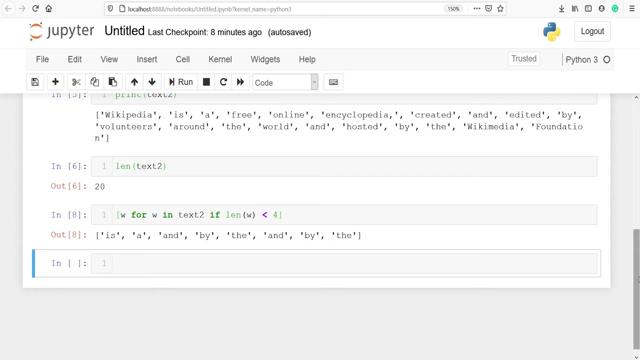 4 length letters and the maximum letter you can see here is 3. this is how you can find a specific length of words and for that we can use the list comprehension. then there is a method: is title, and this will check if the first character is capitalized and the others are. 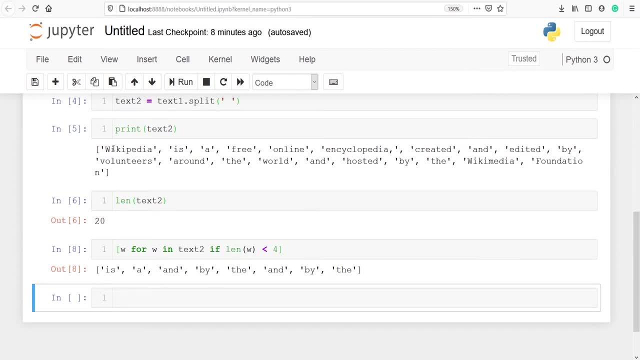 small. for example, here you will see, in Wikipedia the first letter is capital W. here also in wikimedia the first letter W is capital. in foundation also, the first letter F is also capital and we can find all these words using the method is title. I will run a list: comprehension. 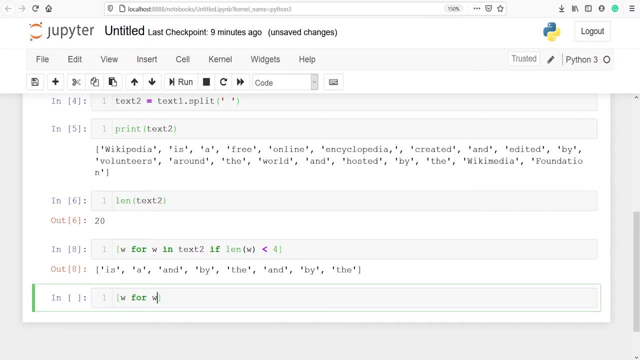 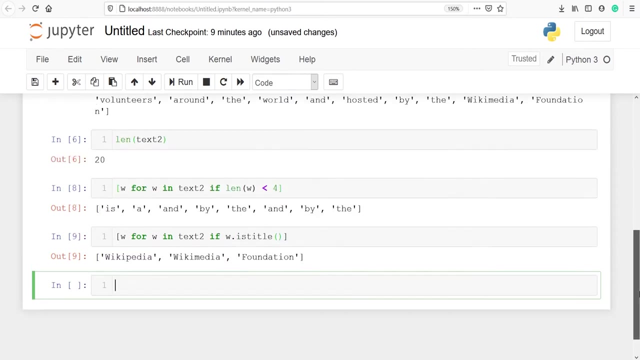 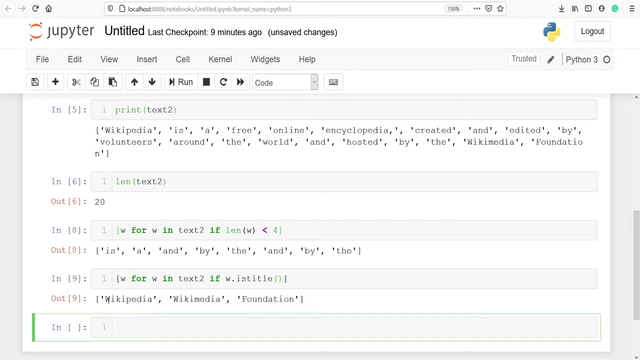 here also I will write W for W in text2 because we are going to check in text2. if W is title, I will execute our code in the output. you can see that we got three results, because these three words are starting with a capital letter. the first letter is capital. here also the first letter is capital. 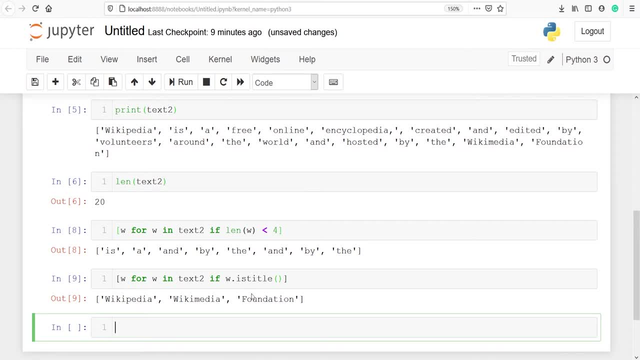 and here also the first letter is capital. using the method is title, we can check any word, if that word is starting with a capital letter or not. next method is ends with. this function is used to find words that ends with a specific alphabet. for example, we want to. 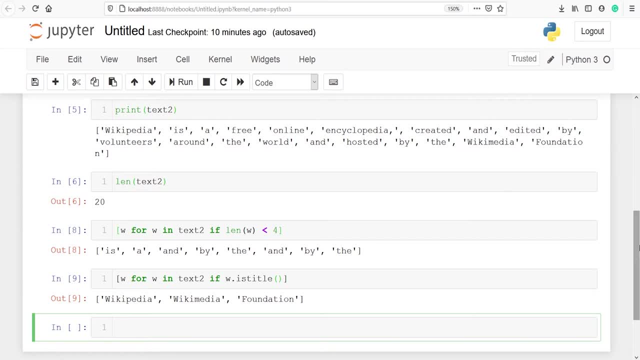 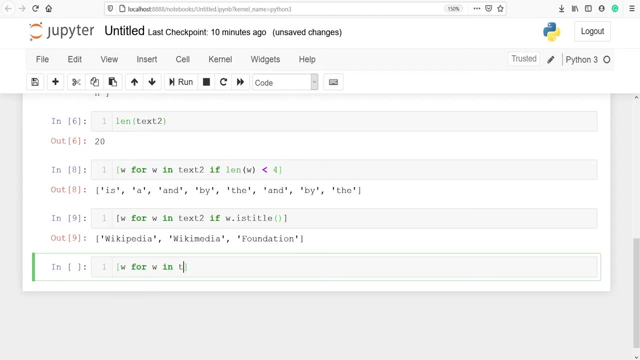 find the words that are ending with alphabet if w in text2. so there is no voodoo type, you know, but there are nohave that are ending with alphabet. if, I will make a list comprehension and I will write a loop W for w in text2. if w, then we will use the function ends with. 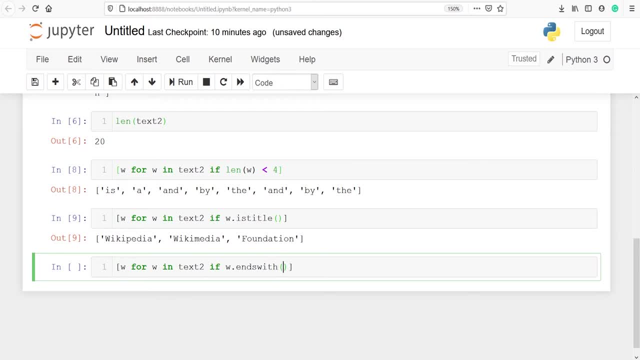 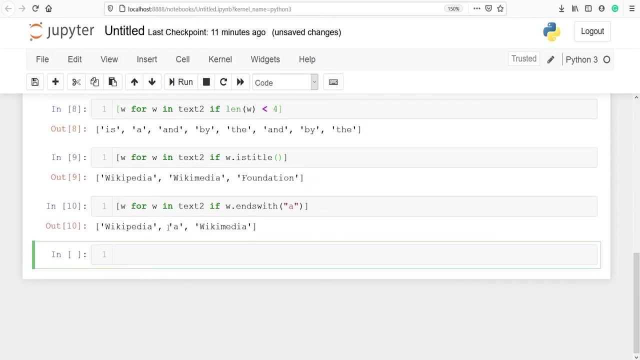 and we will pass alphabet here and we want to check whether a word is ending with the letter. if so, in single-code or double-code you have to type the alphabet. I will typeb here. let's execute the code in the output. you can see that we got result wikipedia. it is ending with: 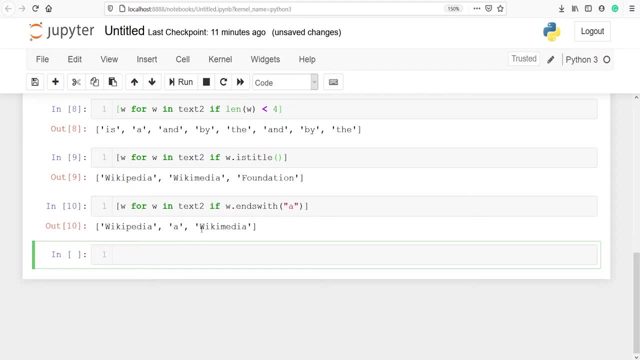 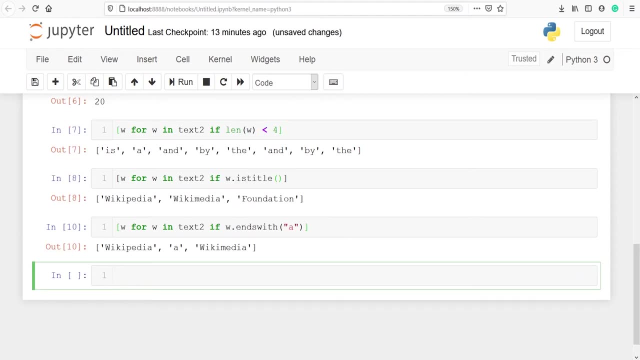 the alphabet a, then we have a itself, then we have wikimedia. this is also ending with a. now we will look at this set function, and set function is used to get the unique values in a sentence. i'll make one variable, text3, and i will write: what is this? what is that? let's execute our code. let's print. 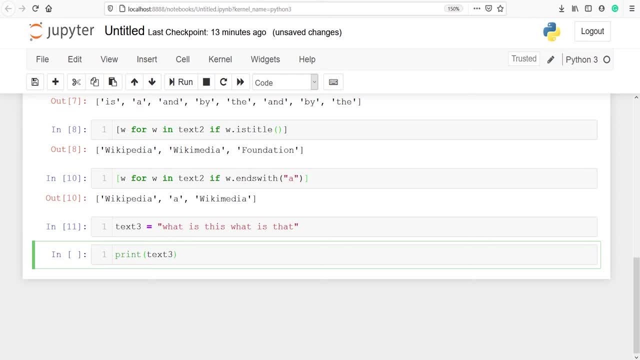 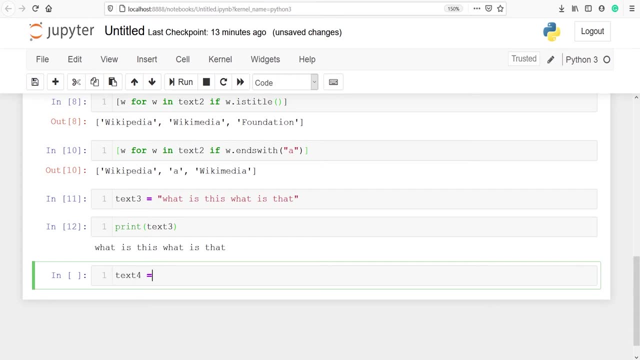 our variable text3. now, first i am going to split this sentence into words. i'll make one variable text4 and then i will call text3 and split. and i want to split on space, so i will type a single code space. let's print our variable text4. 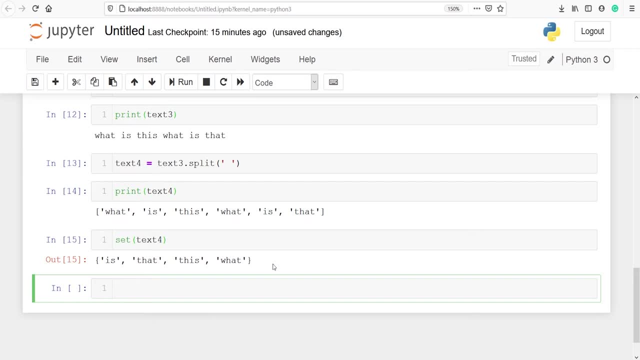 in the output you can see that we got unique words here. in our original variable text4 we have what is repeating twice. here this is the first time and here this is the second time. but using the method set, we got what only once here. so if we want to get the unique elements, we have to use 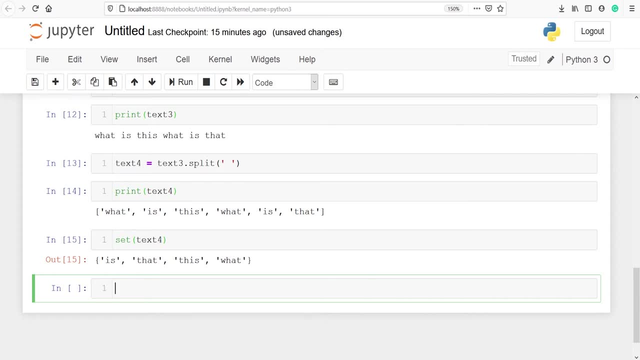 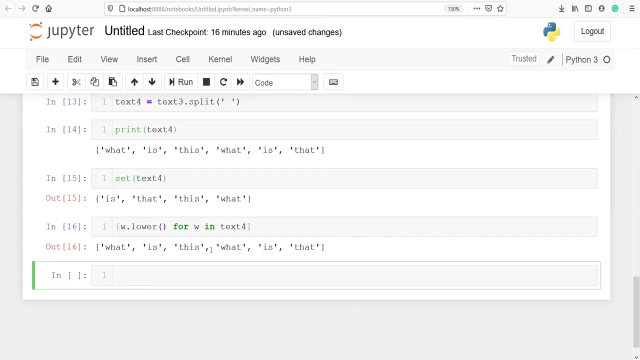 this method set. the next function is lower and this will make all words in lowercase. i'll make a list comparison: w dot lower and this is the method for w in text4. so here in the output you will see we got all the words in the lower case. 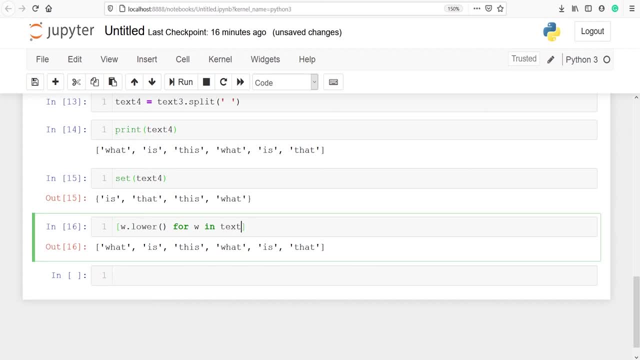 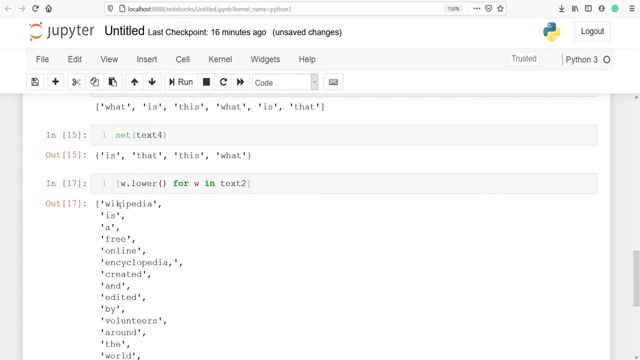 and instead of that i will apply this on text2 and here in the output you will see we got all the words in the lower case. wikimedia ls constparts are repented. we will see all the words in the lowercase. the common Wikipedia also got converted into lower case earlier. the first letter was in capital letter. 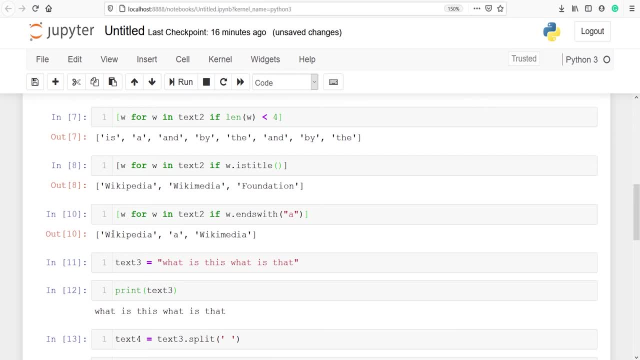 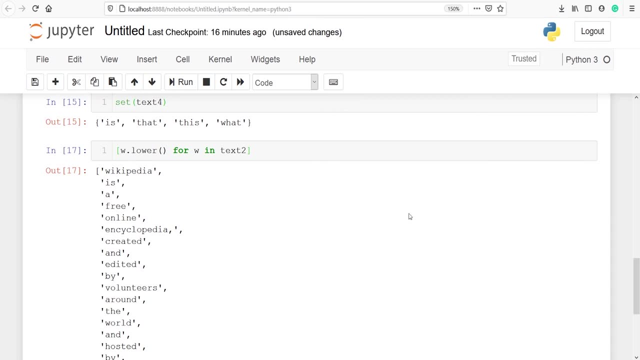 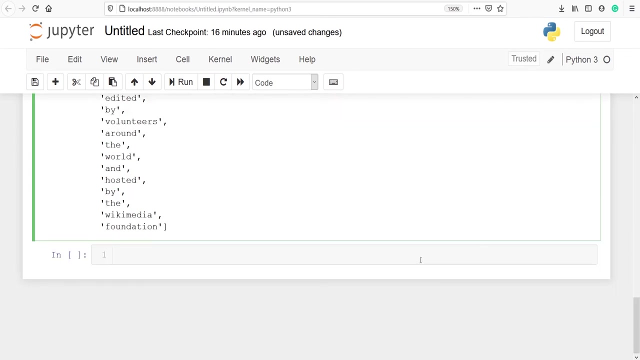 and we can verify from here. here you can see we have the first letter in capital letter. so, using the method lower, we can convert all the words into lower case. similarly, we have upper case. we will copy this code from here, we will paste it here and, instead of lower, 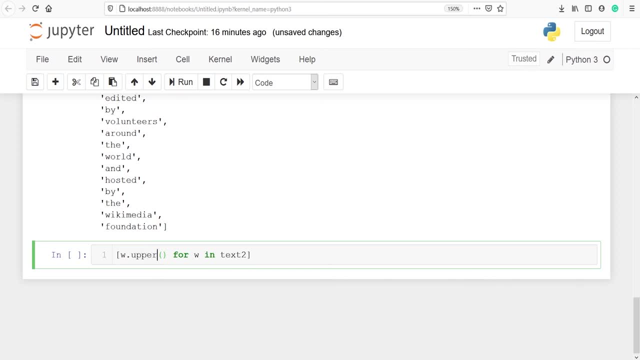 I will call the method upper and this will convert all the words into upper case. let's execute our code. in the output you can see that all the words got converted into capital letters. so using method upper, we can convert all the letters into upper case to get each. 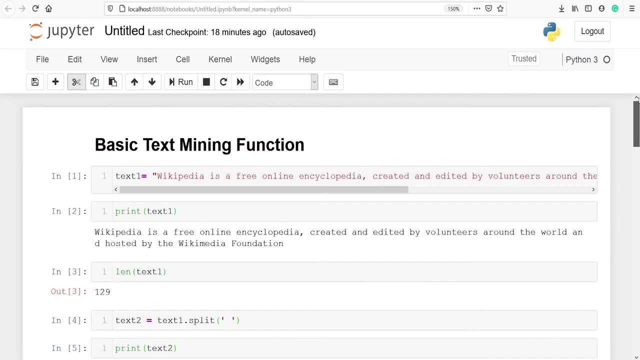 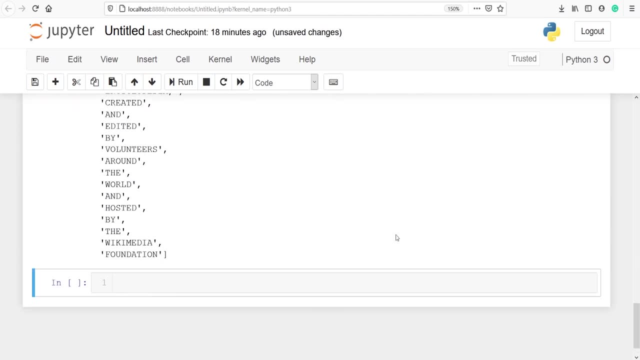 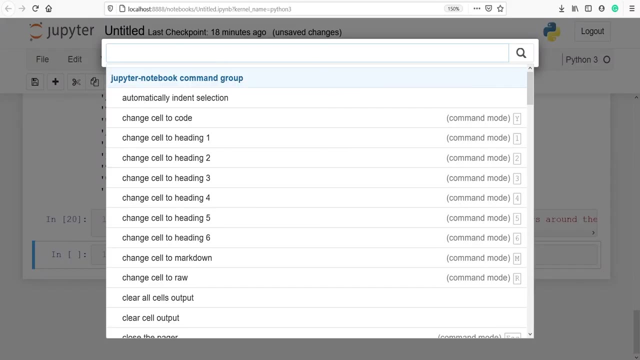 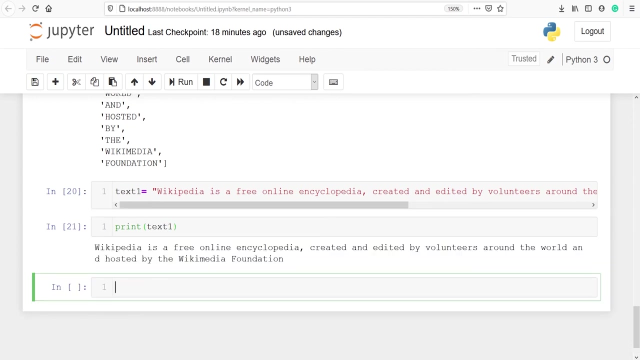 alphabet. we will use the function list. I'll copy this code from here and I will paste it here. let's execute our code. let's print our variable text1. print text1. now I will use the list here. so I will write list of text1 and in the output you can see. 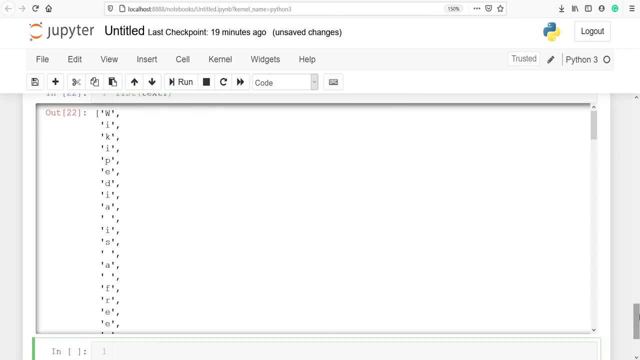 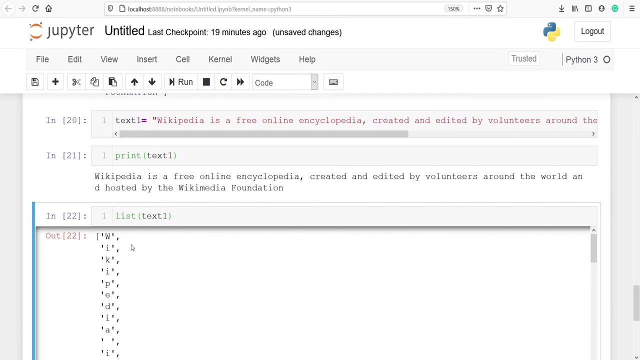 that we got each alphabet. so here we are getting each and every alphabet from the complete sentence. so first is wikipedia. from wikipedia we are getting each and every sentence: w, i, k, i, p, e, d, i, a. so to get all the alphabets you have to use the method list here. this: 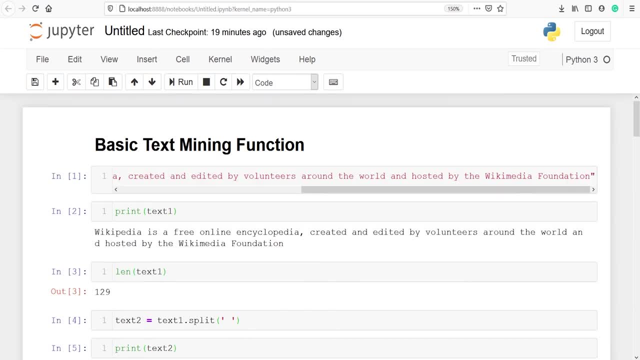 tutorial was about some basic text function in python. I hope you enjoyed this video. if you like my video, please subscribe to my channel. thank you for watching.